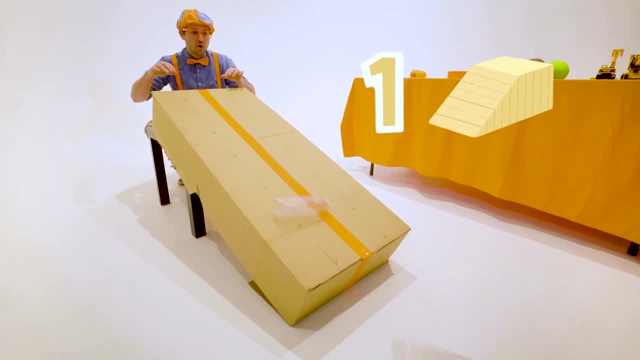 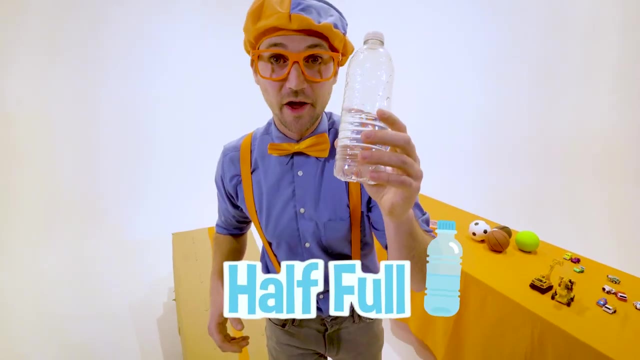 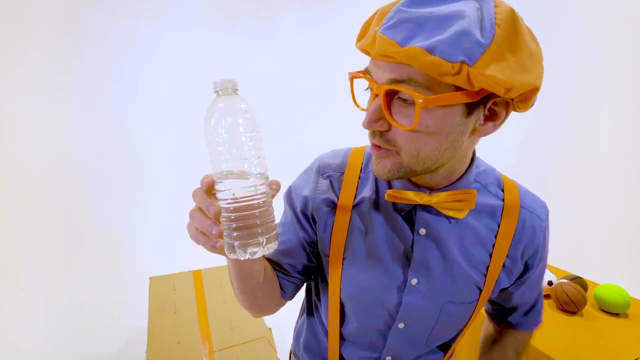 Awesome. Three, two, one, Whoa, Yeah, Wow, Wow, The half full water bottle. Totally, We beat the empty water bottle. How do you feel after your race? half full water bottle, Oh, Blippi, I feel amazing. I can't believe I've won. 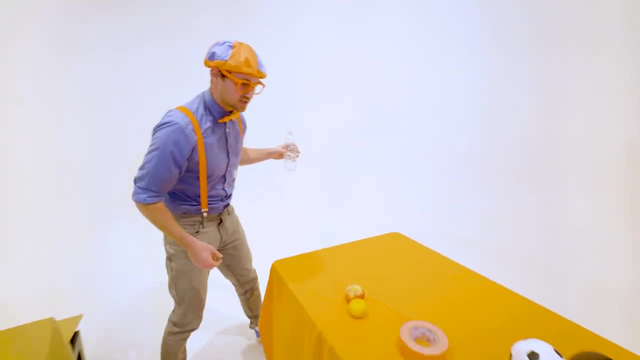 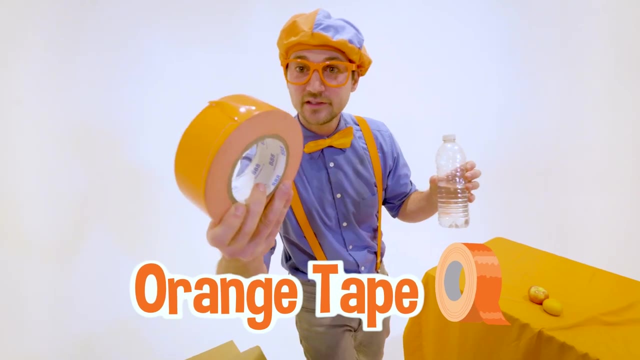 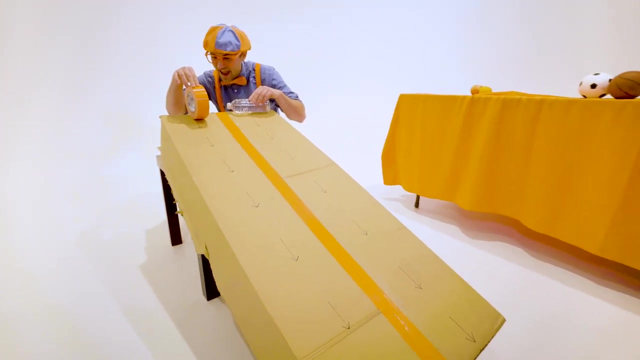 Great. Well, it's going to move on to the next race. Half full water bottle versus extremely bright orange duct tape. Alright, Here we go. Are you ready? Ready to race? Are you ready? You know I'm ready, Alright. 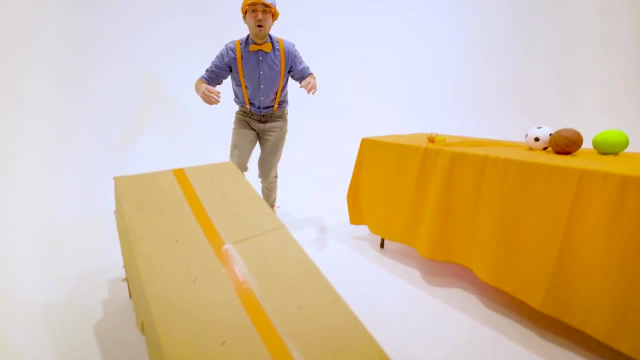 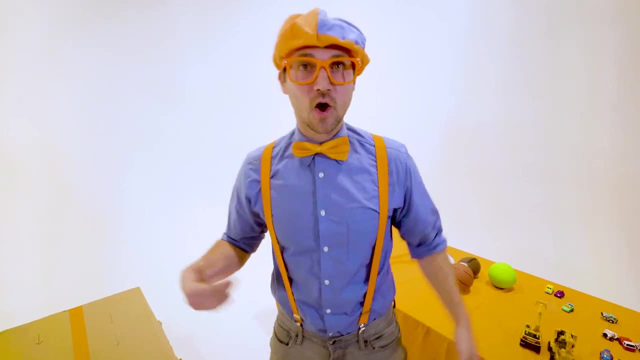 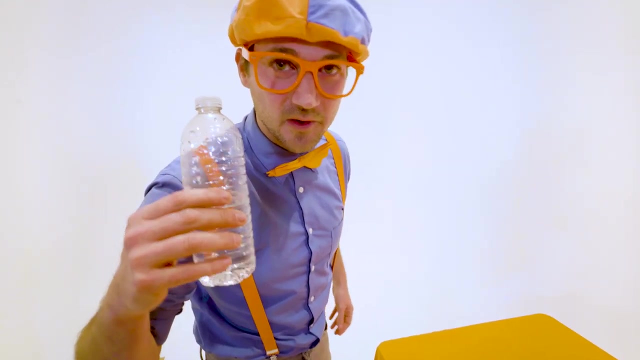 Three, two, one, Whoa, Whoa. Did you see that? Yeah, The water bottle rolled down Way to the bottom Way quick, Way faster than the duct tape. Perfect, So now it can move on to the next round. 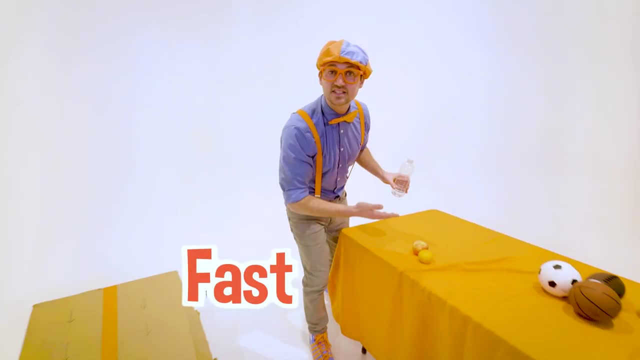 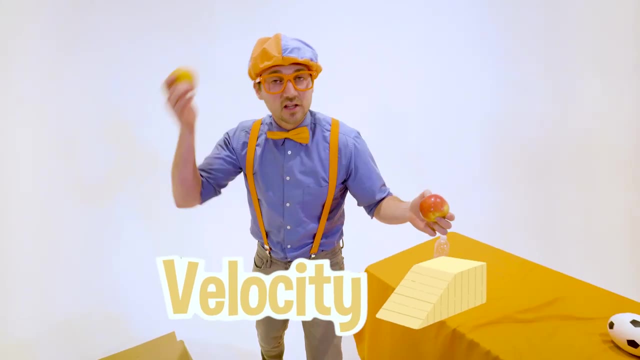 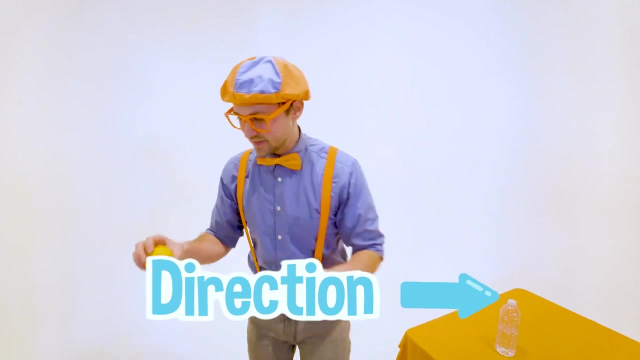 Have you ever wondered why these items some go fast and some go slow? Yeah, It's because their velocity. Yeah, Velocity is basically, It's basically the speed at which they're rolling down, The speed and the direction. Yeah, There's a lot of things that actually determine what the items. velocity is. 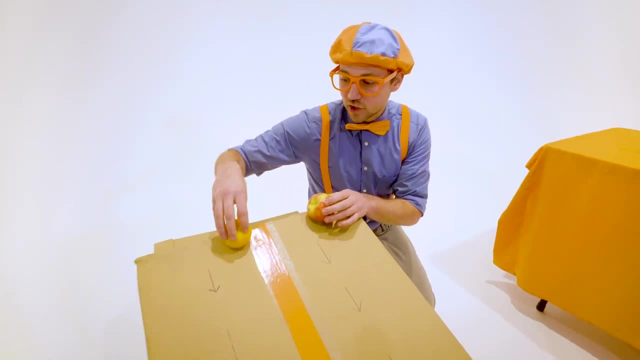 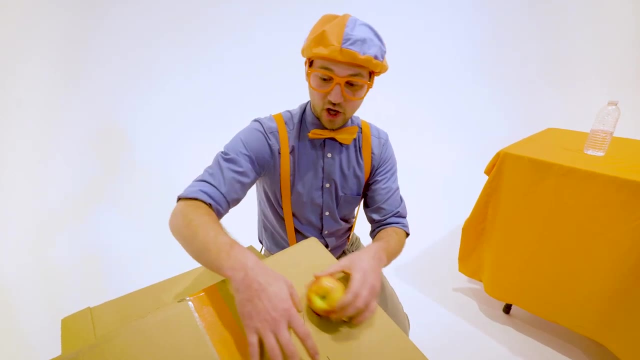 I mean, like, think about it like this: There could be a lot of friction and it like can't slide, or maybe it rolls, compared to you know, maybe they're sharp edges. There's just so many things that you know determine how fast. 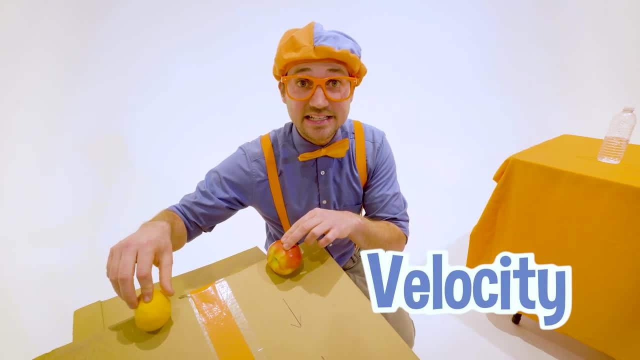 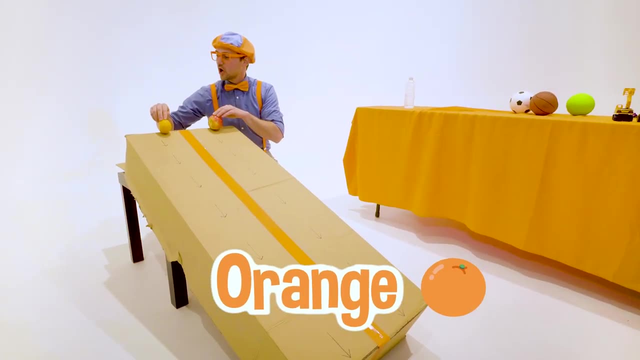 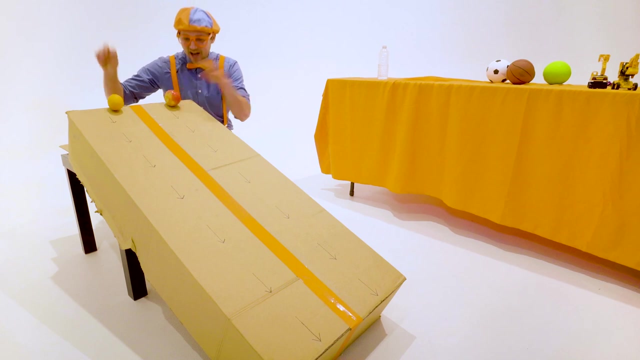 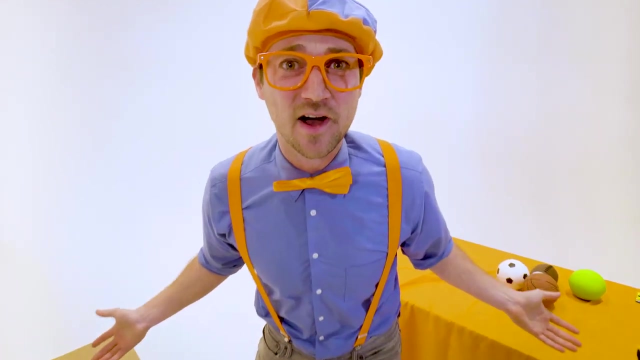 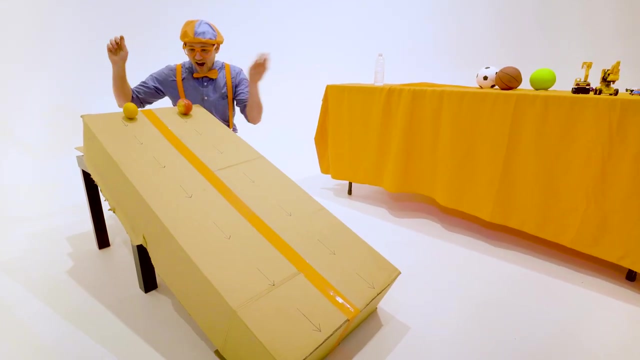 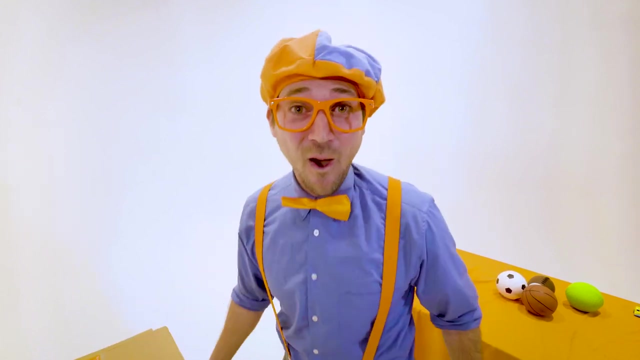 How fast, How much velocity these items have. so let's let these two items go. We have orange over here and apple over here and let's see They were actually really close to each other. no one, let's see that instant replay. Oh, Awesome, all right, let's pick two more items. 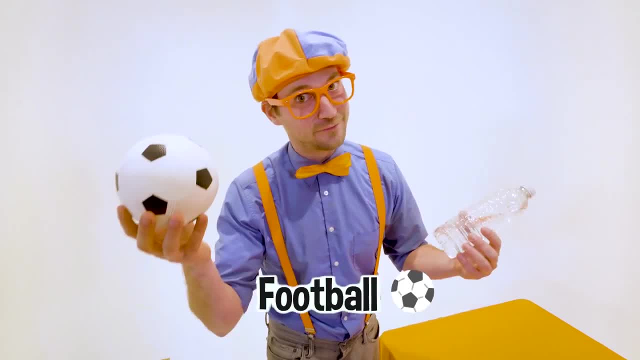 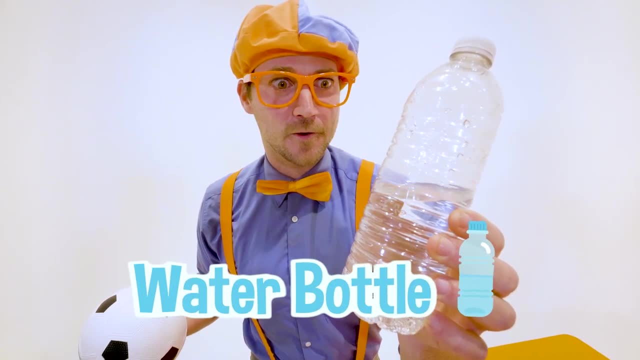 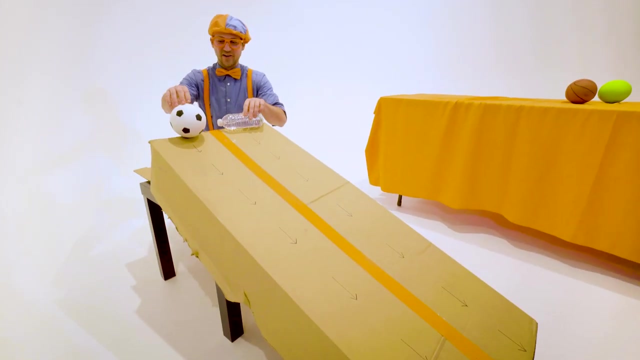 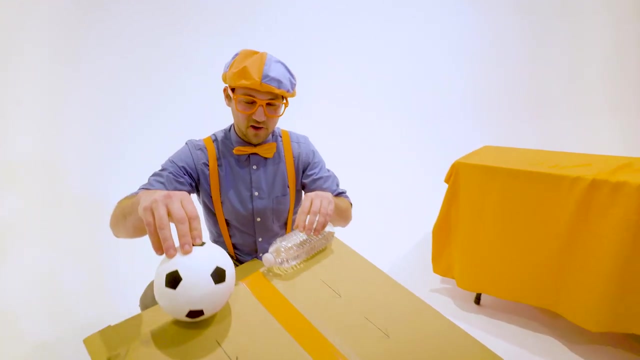 we have a soccer ball or a football, depends where you live, and the Half-full water bottle. the champion, Okay, Wins. all right, here We go. Are you ready? I'm good to go. Are you ready? I was born already? all right and away we go. 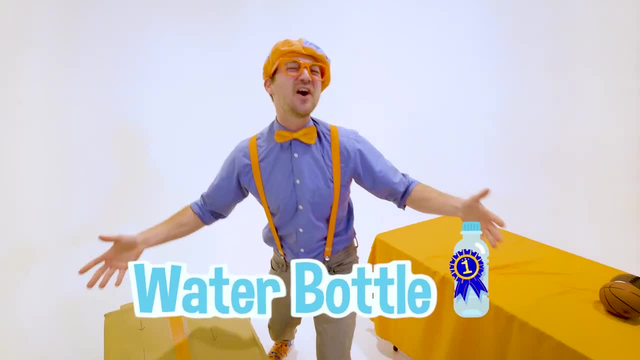 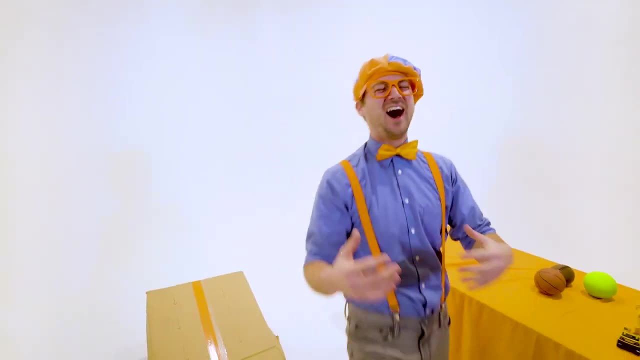 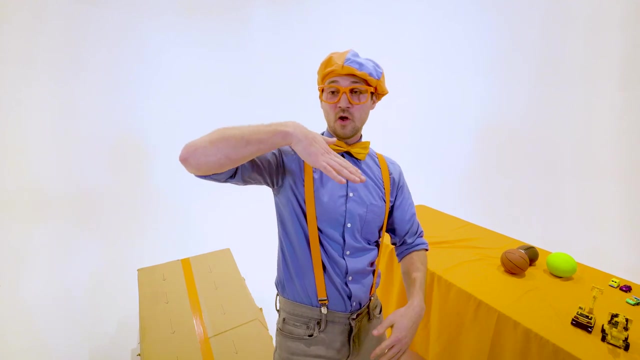 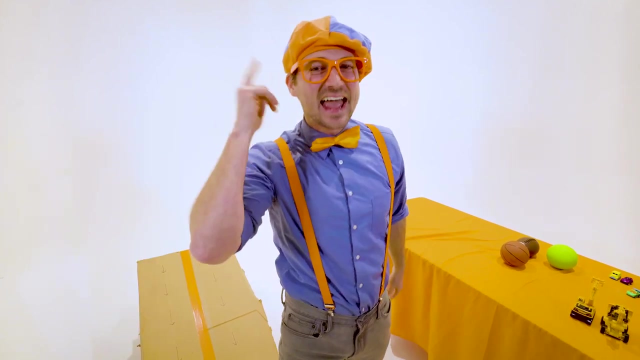 Not believe it. the half-full water bottle wins the velocity race Goes. Wow, that was awesome learning about velocity and Fast that water bottle went and how the ramp is angled. But yeah, if the ramp was flat it definitely wouldn't go anywhere, right, Yeah, Hey, can you think of a machine that is actually really fast? 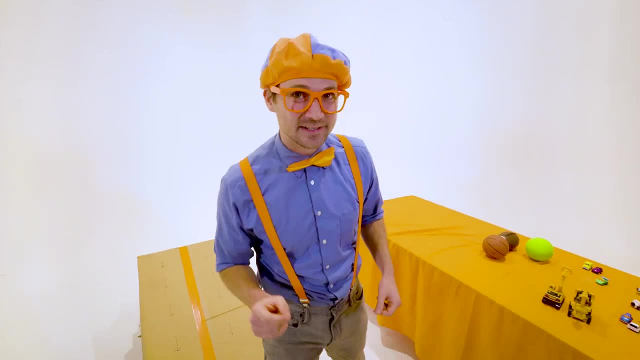 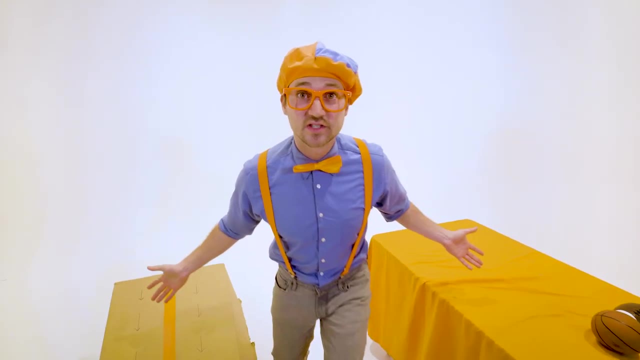 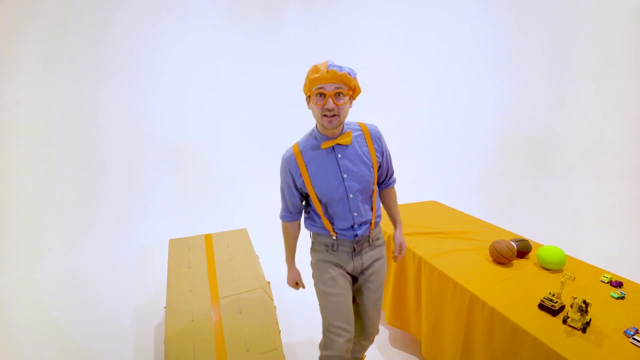 Yeah, there's a lot of them. Okay, Let me give you a hint. Okay, this machine does not go on the ground. Well, it does, but then it goes in the air. Yeah, Whoa, I hear one. Yeah, maybe you've got to fly in one before. 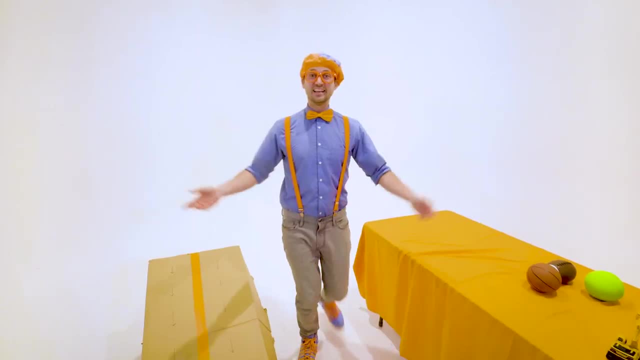 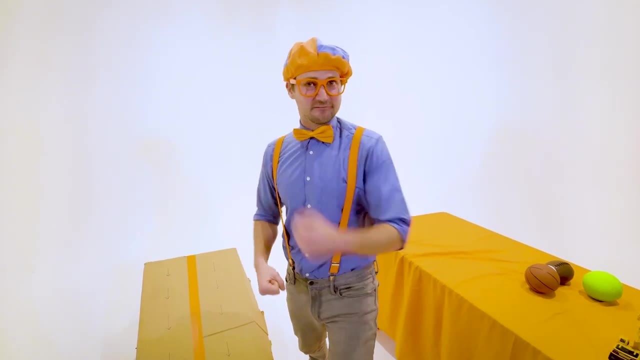 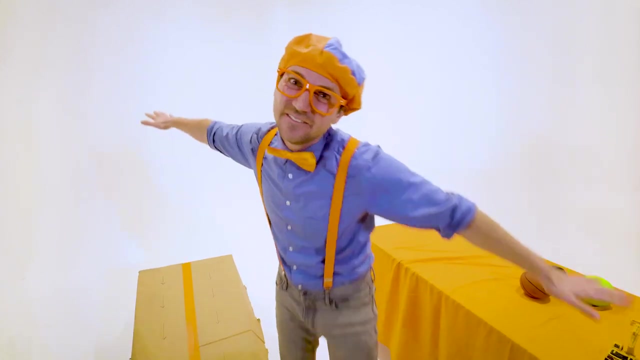 Fly- yeah, they fly in the air. Yeah, airplanes- Yeah, airplanes are really fast. and, speaking of speed and velocity, I think you and I should watch the airplane video. Yeah, airplanes are really fast and I think you and I should watch the airplane video. I think you and I should watch the airplane video. 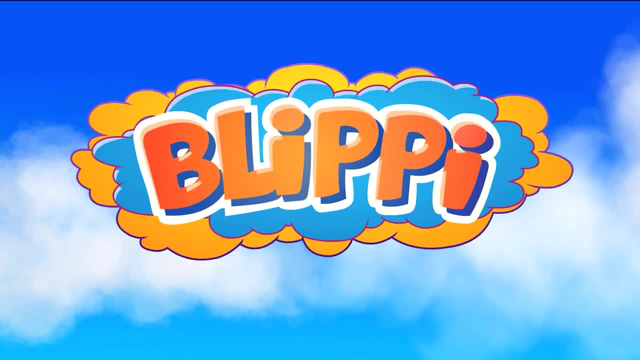 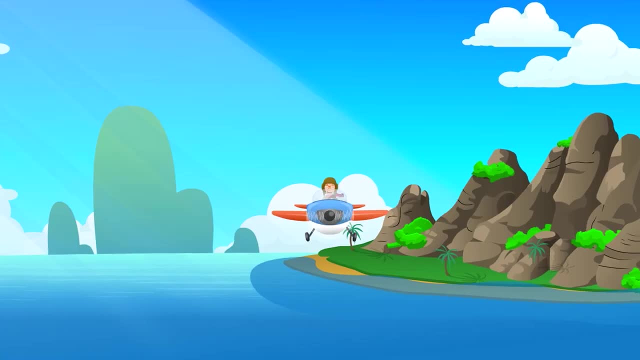 but I think you're gonna be like me. Yeah, I was like you like me. Oh, this thing is cool. Oh yeah, Hey, did you ever fly here? No, no, I didn't. But maybe in the next few years, if you go back, you'll be like it's a dream. 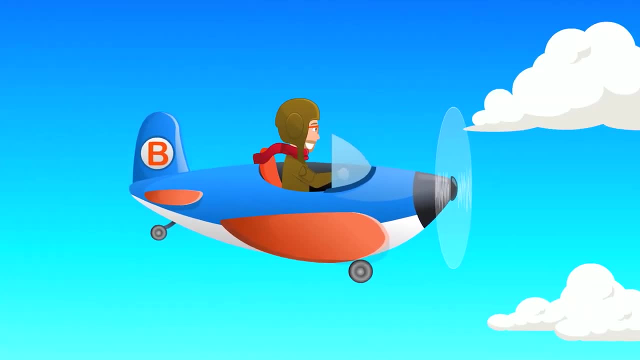 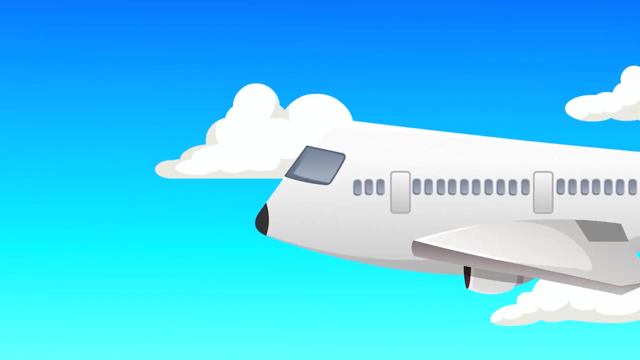 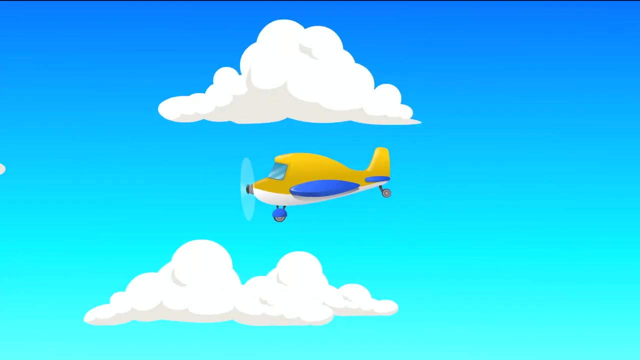 Yeah, but you're gonna scared, We're gonna fly somewhere else, I think. so, yeah, let's do a little bit more. Yeah, I mean like you're gonna fly in that way. Yeah, I'll fly with you. big as a building, some are small as a car. that's amazing. some airplanes transport people, some fly. 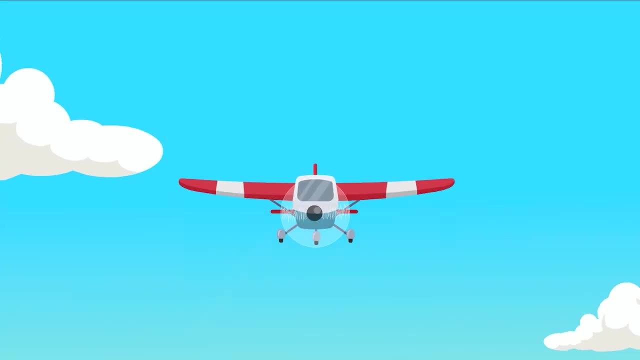 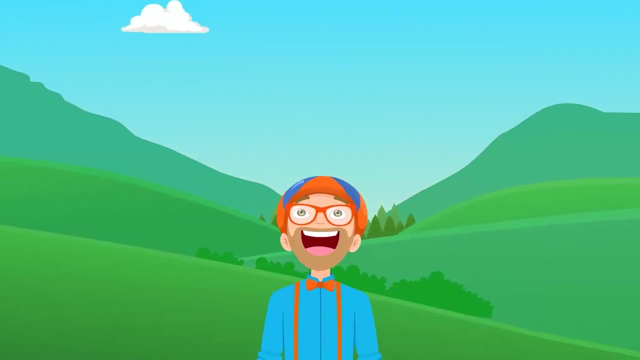 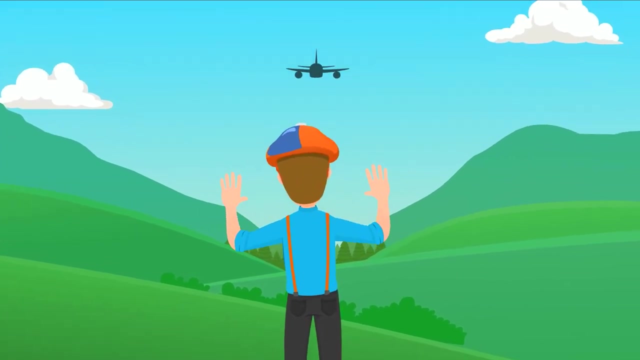 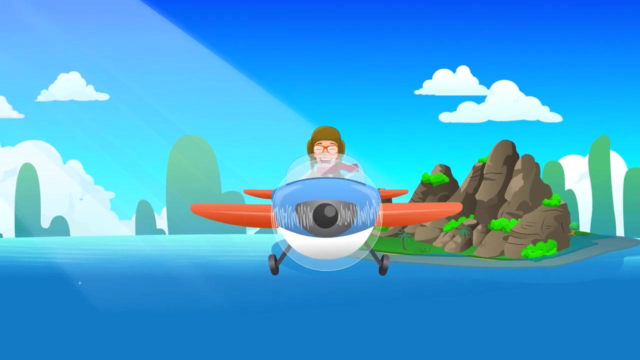 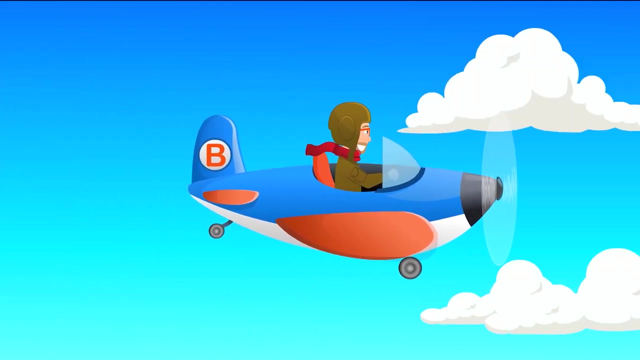 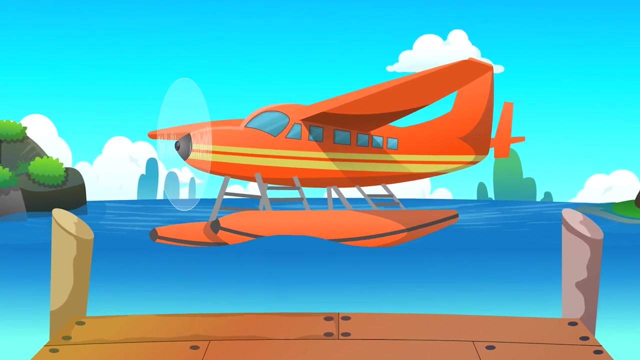 near to the stars. some airplanes fly with propellers. some airplanes fly with jet engines. I love to look up and see their wings waving down at me. airplanes, airplanes flying all around the sky. airplanes, airplanes flying way up high. some airplanes can land on water, the most land. 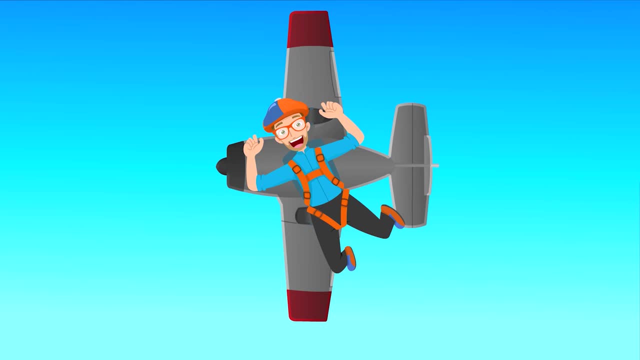 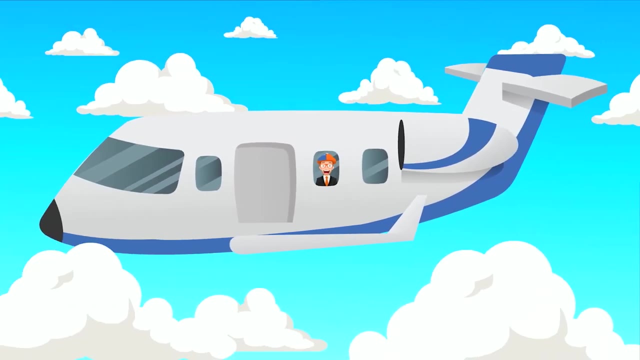 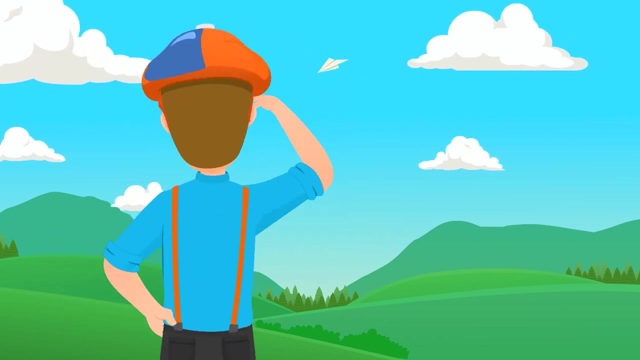 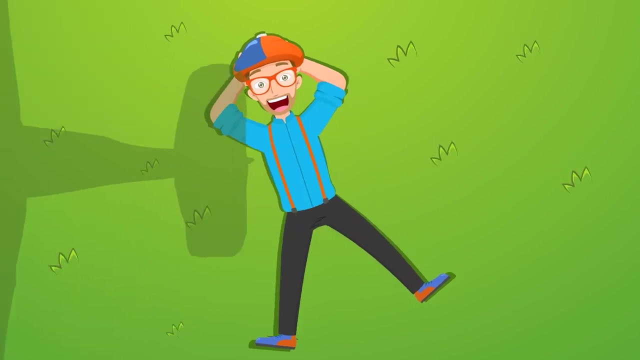 on landing strips. so versatile. some airplanes fly just for fun, some fly for business trips. business or pleasure, you can make an airplane out of paper, throw it in the air and watch it go. I love to look up and see its wings waving down at me. airplanes, airplanes. 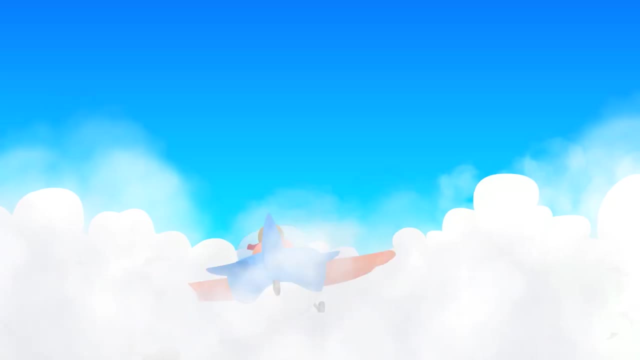 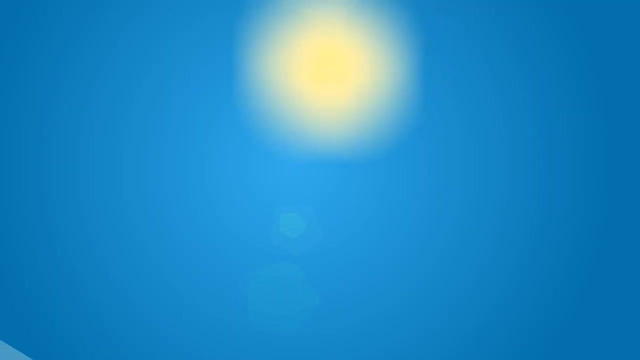 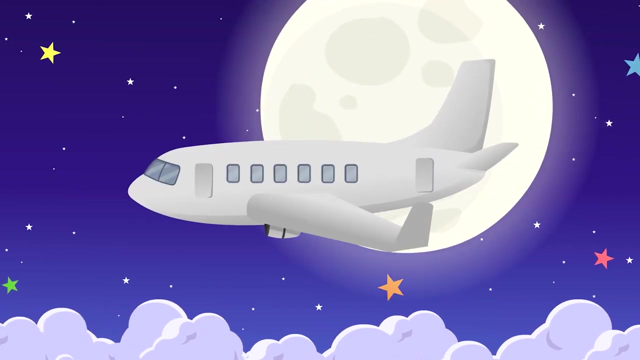 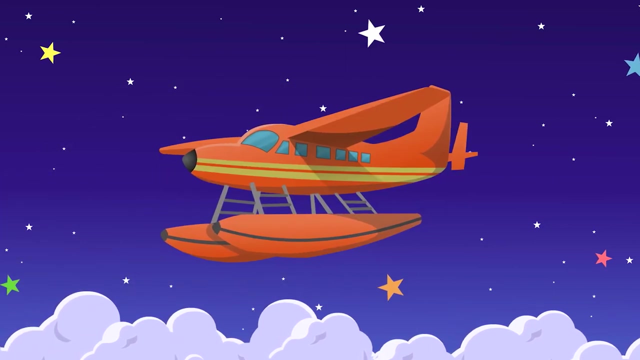 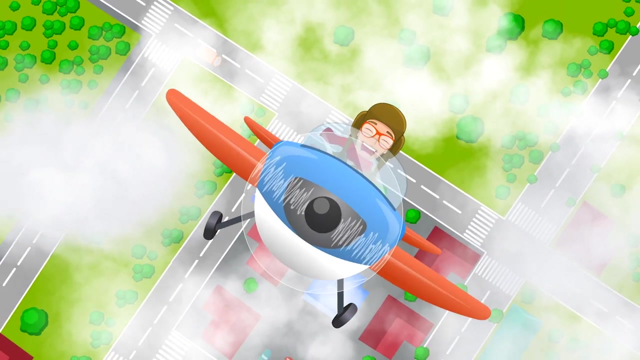 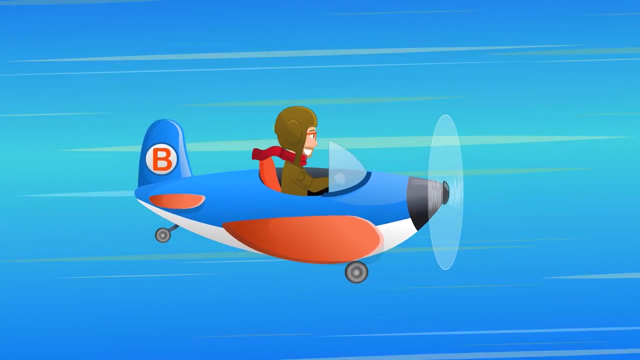 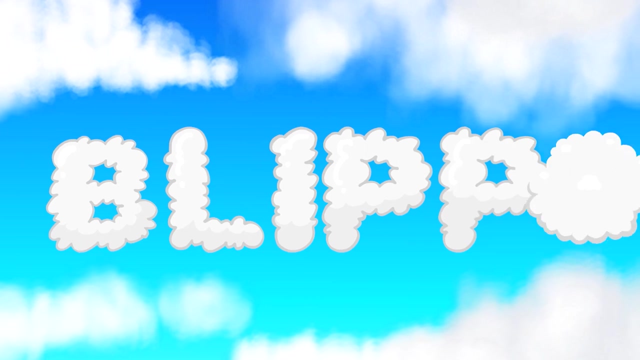 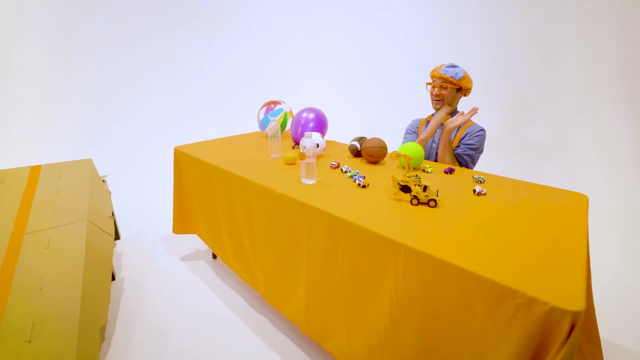 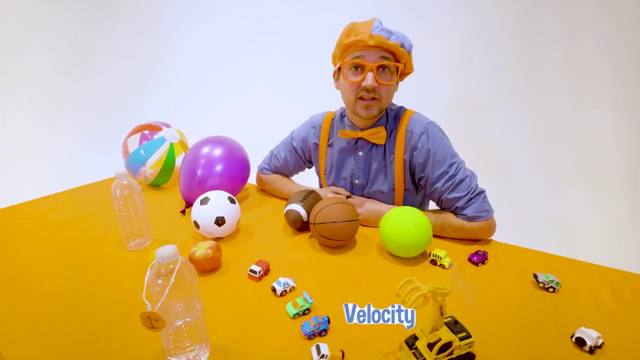 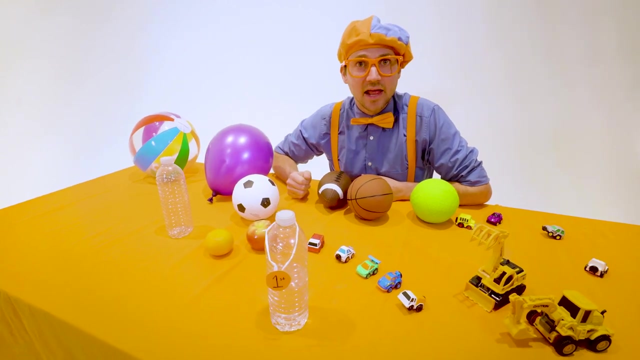 airplanes flying all around the sky. airplanes, airplanes flying way up, high airplanes. airplanes, airplanes flying all around the sky. airplanes, airplanes flying way up. wow, that was so much fun learning about philosophy with you and it was really fun seeing all these great items compete at the great blippy velocity. 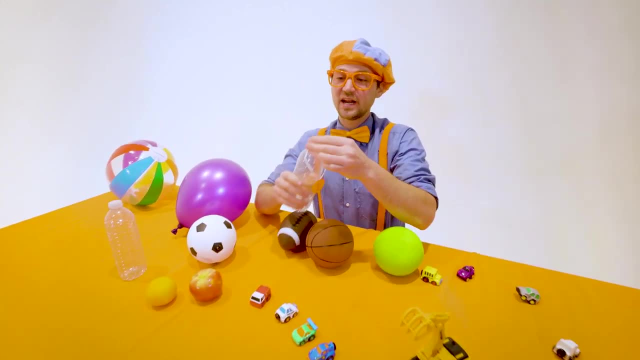 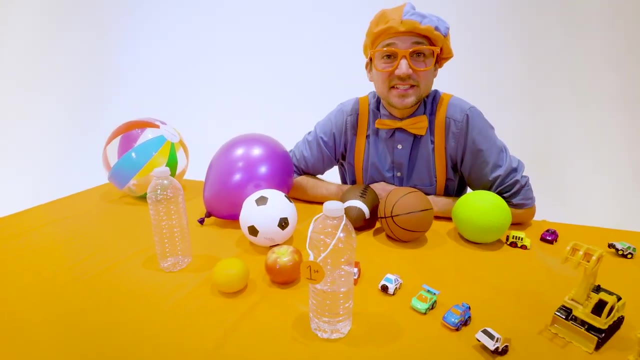 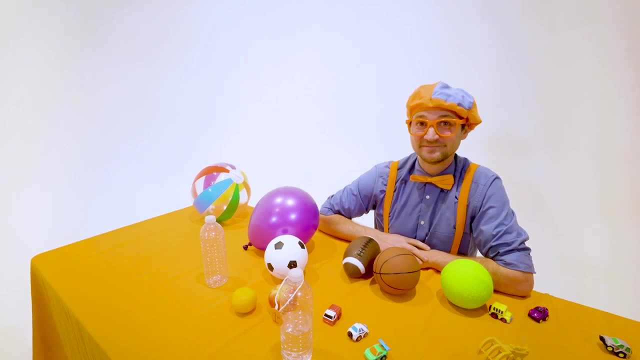 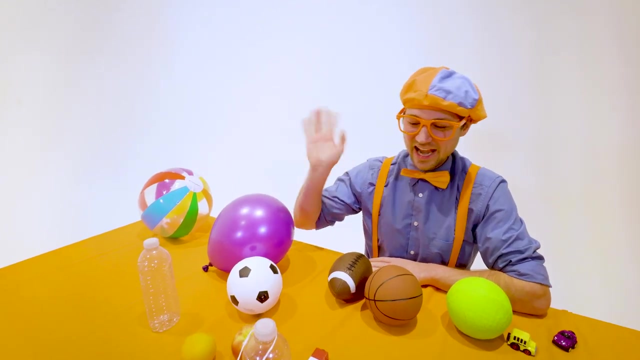 race, haha, but there's only one champion, and today that was water. wow. well, this is the end of this video, but if you want to watch more of my videos, all you have to do is search for my name. will you spell my name with me? b-l-i-p-p-i. blippy. good job, all right, see you again, buh-bye.